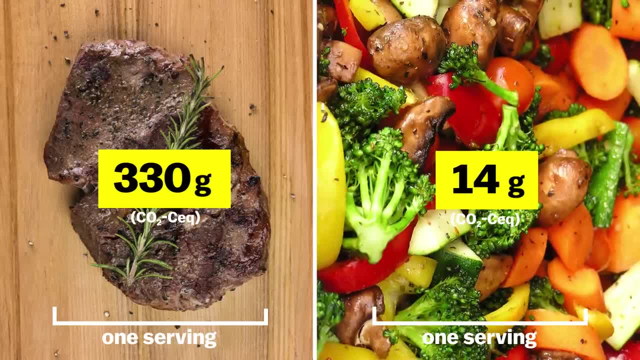 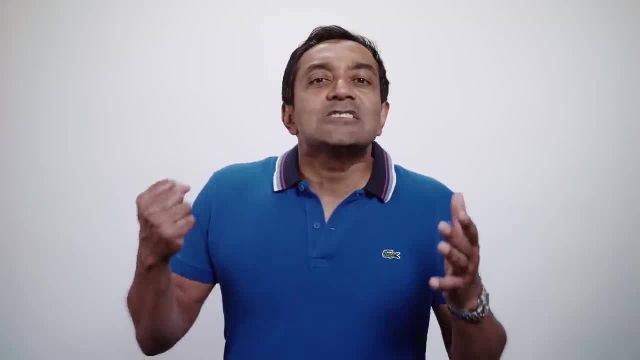 go down even more. Now look at veggies. If I swapped beef out entirely for lentils, well I'm down to practically nothing. So why does beef- and lamb too, for that matter- pack such a powerful punch to the planet? 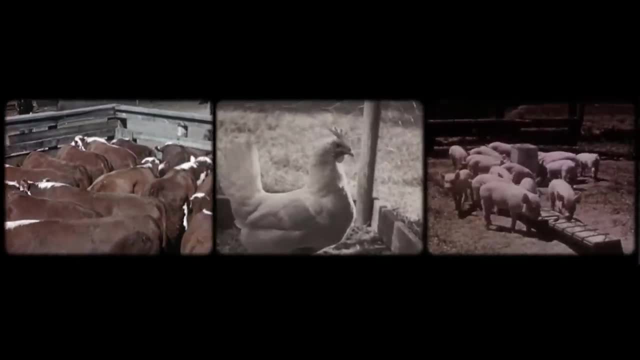 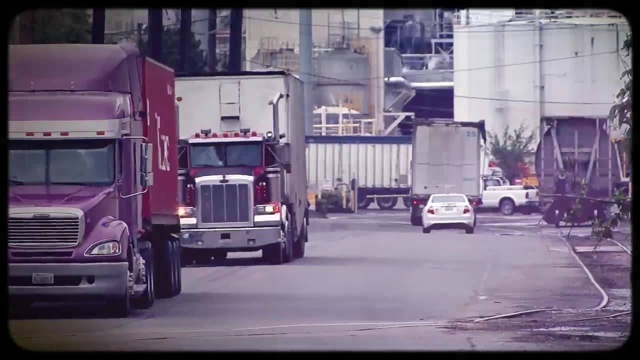 If you're looking for a little over 14% of global greenhouse gas emissions, if that sort of seems low to you, consider it's about equal to transportation. We're talking all the cars, trucks, planes, trains and ships on the planet combined. This is partly because ruminant animals 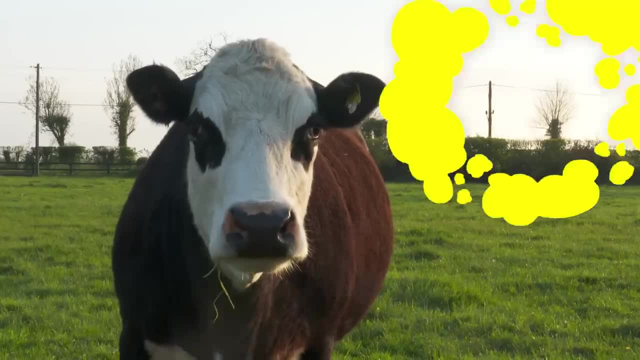 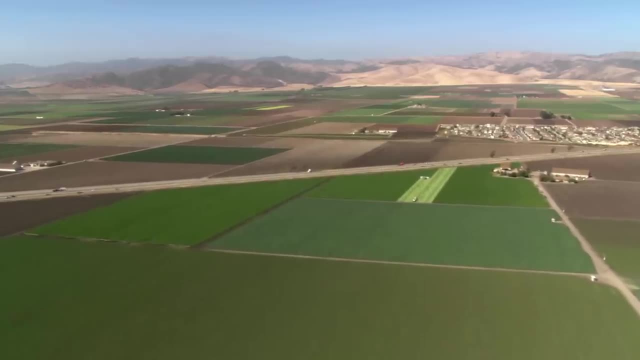 like cows and sheep. they're just gassy, And the methane they produce is at least 25 times more potent than carbon dioxide. Plus, it takes a lot of land fertilizer and about a billion tons of grain to feed all that livestock. 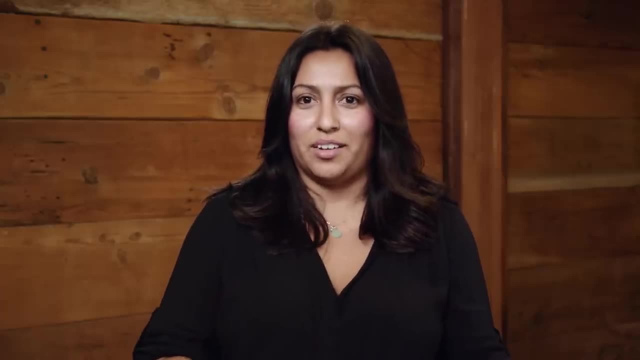 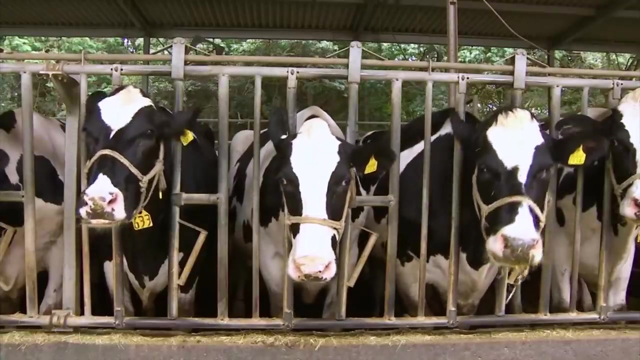 And you could feed 3.5 billion people with that grain. If we were just directly eating these grains ourselves, it would eliminate a lot of the CO2 that's emitted from cattle production. So it's clear that meat has a pretty big carbon load, But it's also worth remembering that not 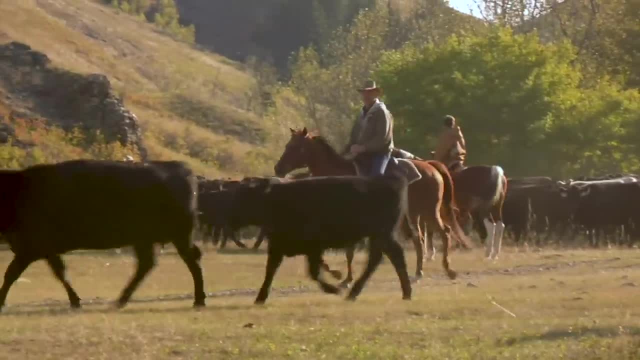 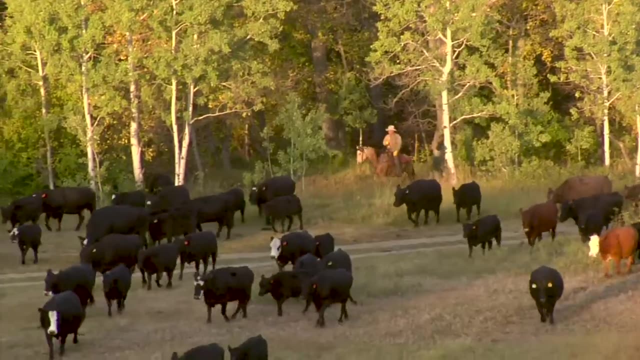 all livestock is raised equally. In parts of the American West, for instance, ranches are working to raise livestock in ways that actually help restore the land, And they're experimenting with ways that soil and grasslands can be used to keep carbon pollution out of the air. But even these 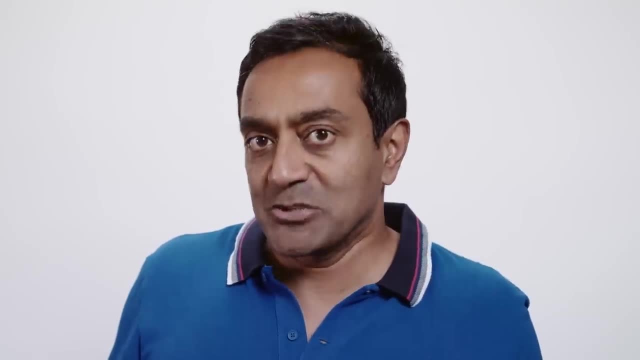 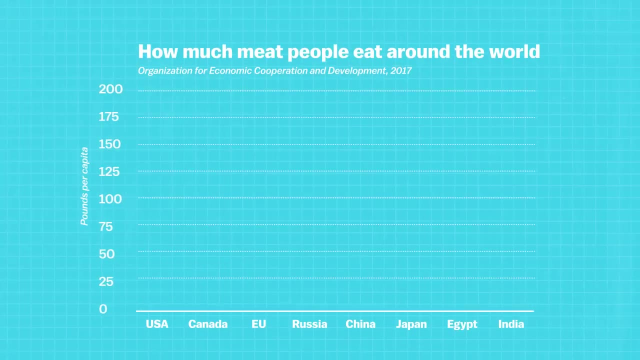 sustainable ranches will really tell you we're probably eating too much meat. I know a lot of people who, if you don't serve them meat for lunch or dinner, they're kind of like: well, when is the meat coming out? It's to the point now where the US actually has one of the highest meat footprints per capita. 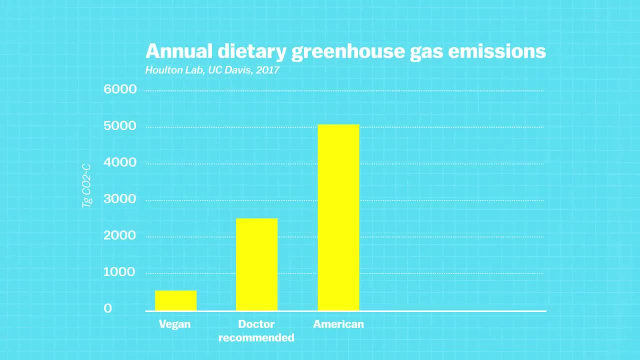 So what about not eating meat at all? Vegan is the way to go for the least impact on the planet, But it's not that much different in terms of emissions than, say, a vegetarian diet. A team found that the environmental impact of the Mediterranean diet is pretty similar to vegan. 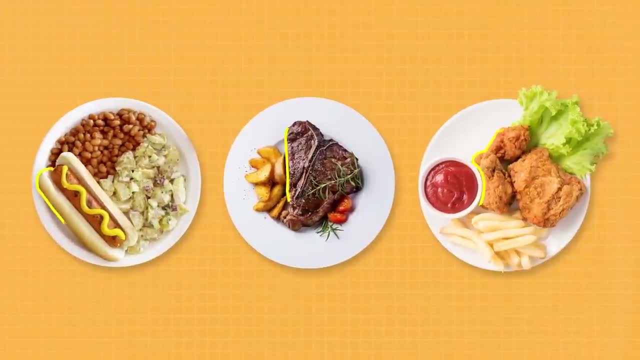 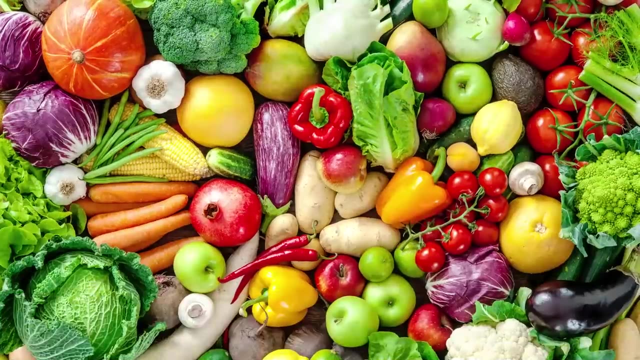 and vegetarian diets. It's a lot less meat-heavy than what Americans are used to. So: fish and poultry a few times a week, beef maybe once a month, plenty of plant-based foods and, of course, loads of olive oil. Eliminating like 90% of your meat intake is more important than